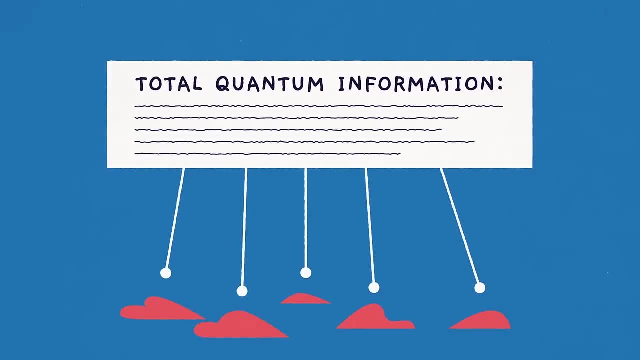 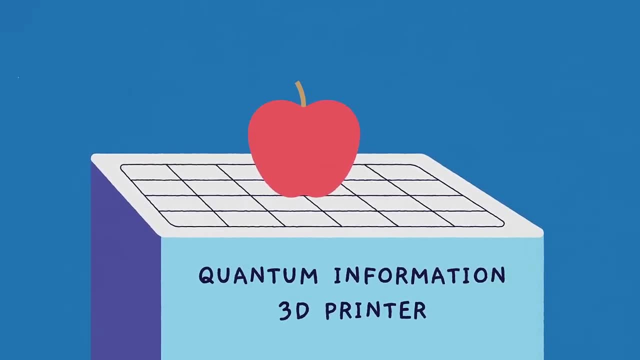 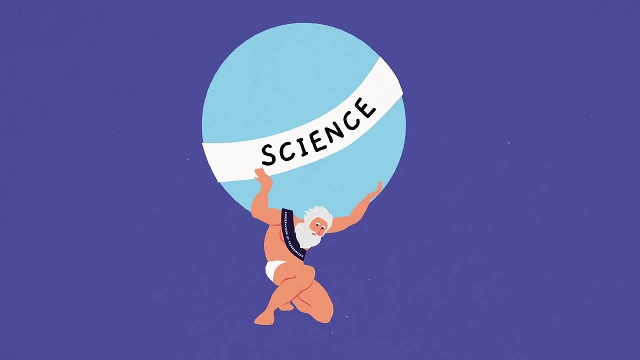 its quantum information is never permanently deleted And, theoretically, knowledge of that information would allow us to recreate the object from its particle components. Conservation of information isn't just an arbitrary rule, but a mathematical necessity upon which much of modern science is built. 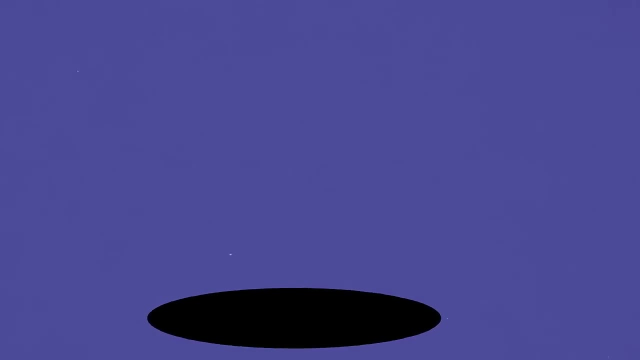 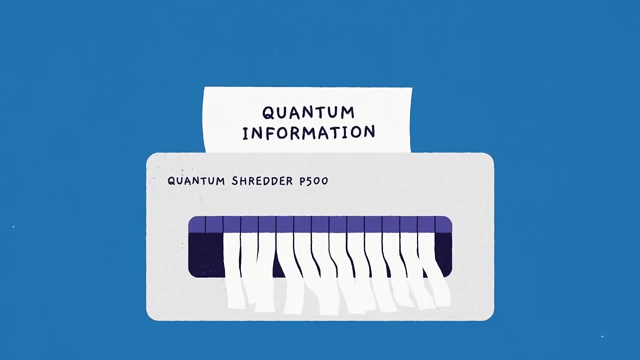 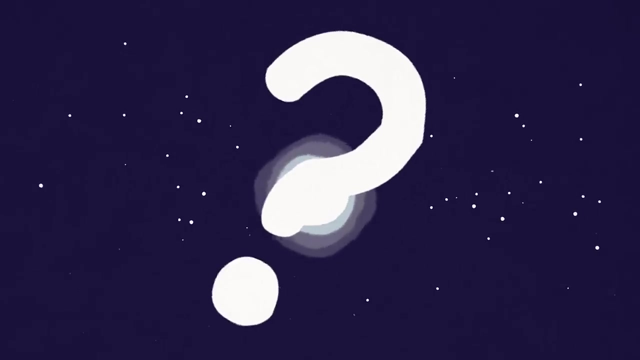 But around black holes those foundations get shaken. When an apple enters a black hole, it seems as though it leaves the universe, and all its quantum information becomes irretrievably lost. However, this doesn't immediately break the laws of physics. The information is out of sight. 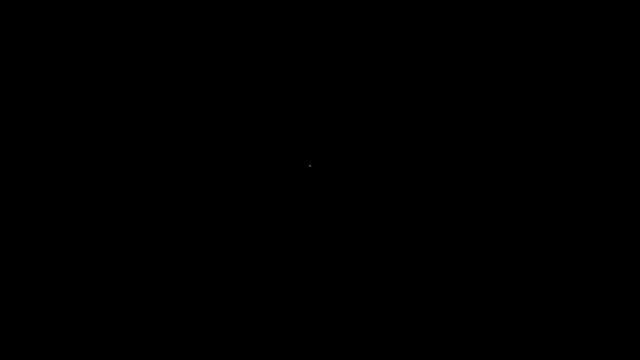 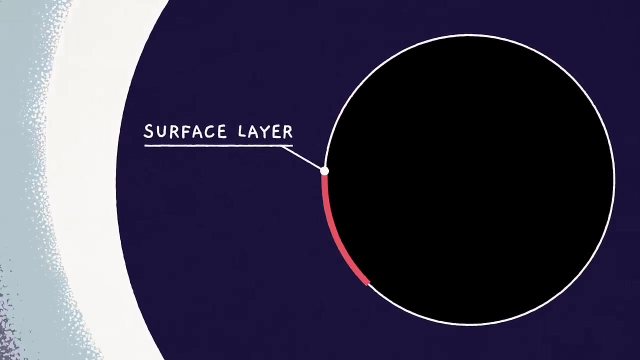 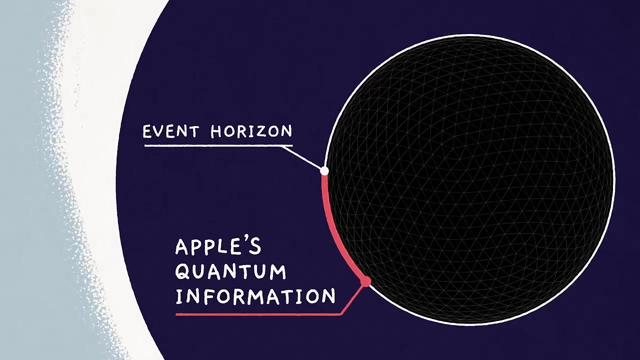 but it might still exist within the black hole's mysterious void. Alternatively, some theories suggest that information doesn't even make it inside the black hole at all. Seen from outside, it's as if the apple's quantum information is encoded on the surface layer of the black hole. 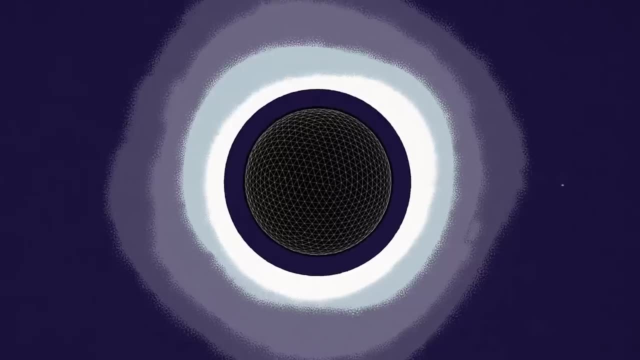 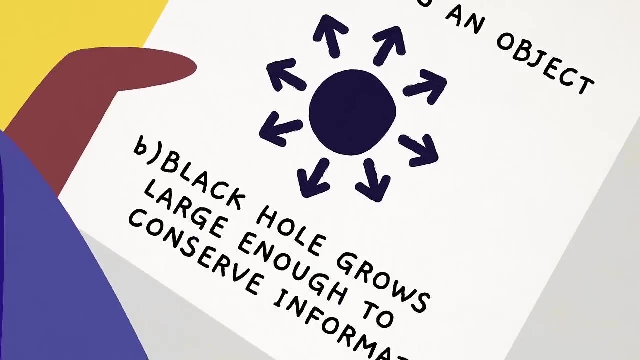 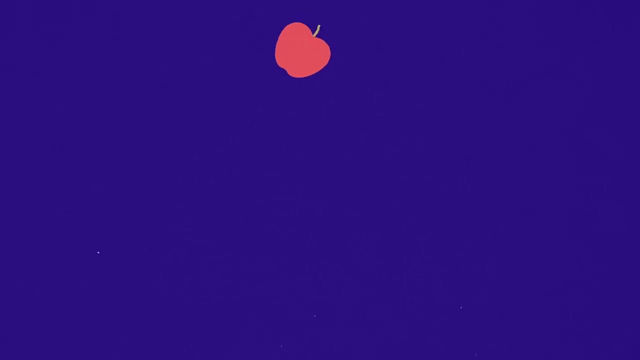 called the event horizon. As the black hole's mass increases, the surface of the event horizon increases as well. So it's possible that as a black hole swallows an object, it also grows large enough to conserve the object's quantum information. But whether information is conserved inside the black hole or on its surface, 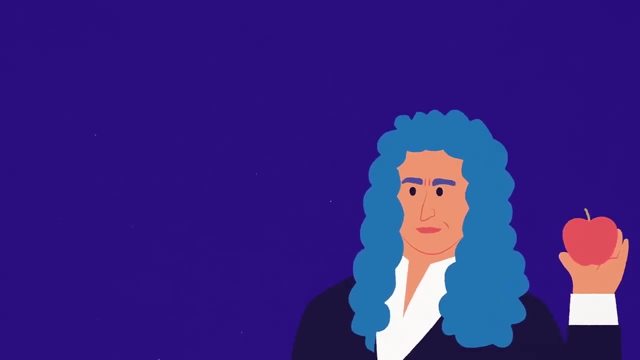 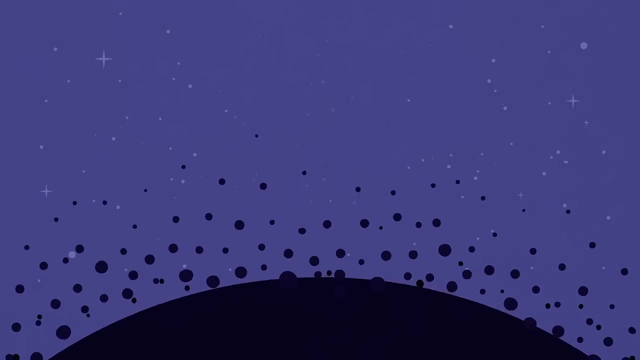 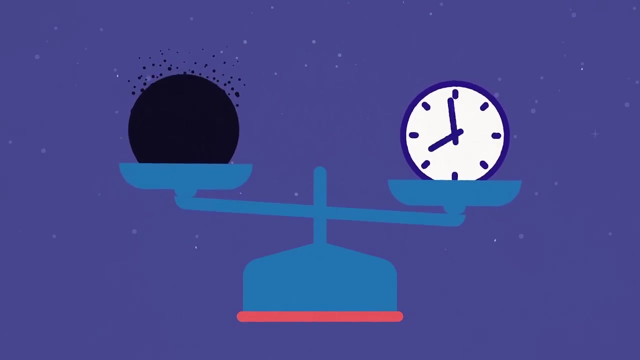 the laws of physics remain intact— until you account for Hawking radiation, Discovered by Stephen Hawking in 1974, this phenomenon shows that black holes are gradually evaporating Over incredibly long periods of time. black holes lose mass as they shed particles away from their event horizons. 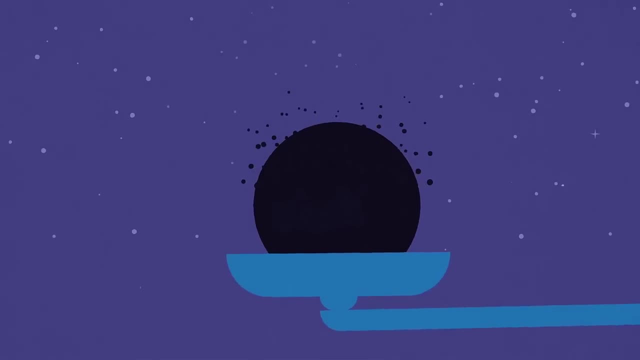 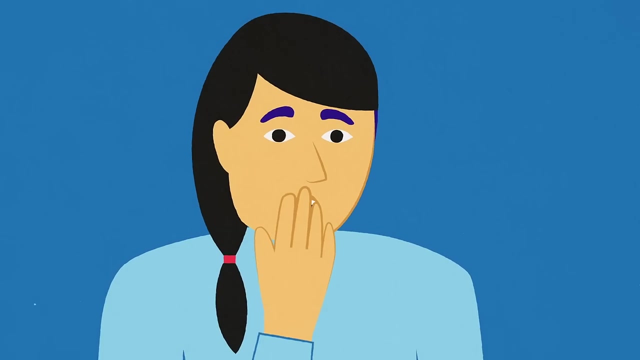 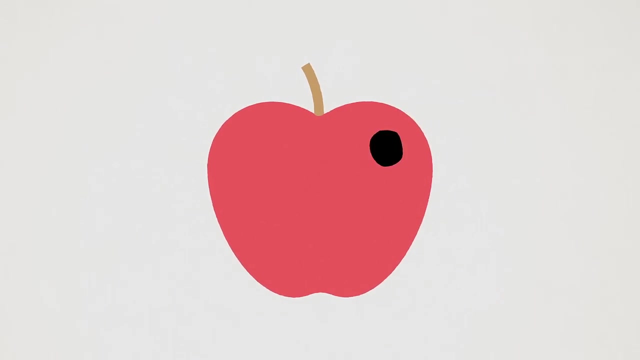 Critically. it seems as though the evaporating particles are unrelated to the information the black hole encodes, suggesting that a black hole and all the quantum information it contains could be completely erased. Does that quantum information truly disappear? If not, where does it go? 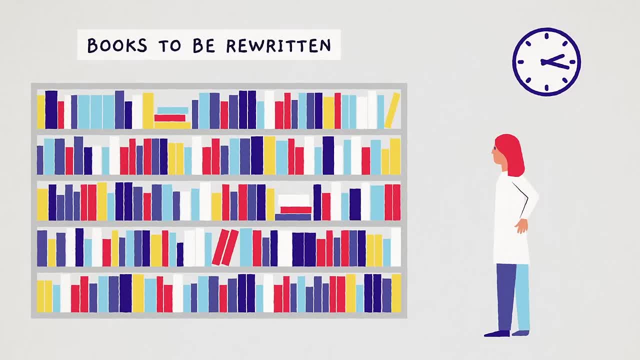 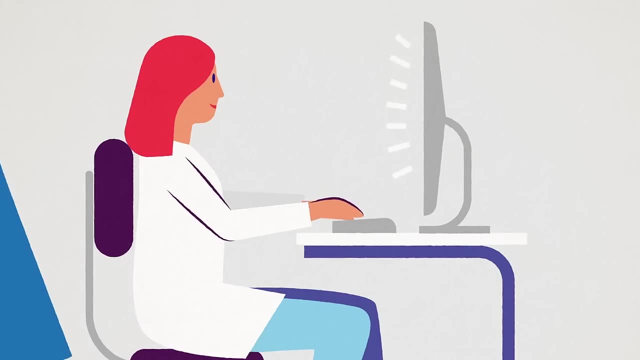 While the evaporation process would take an incredibly long time, the questions it raises for physics are far more urgent. The destruction of information would force us to rewrite some of our most fundamental scientific paradigms, But fortunately, in science, every paradox is an opportunity for new discoveries.